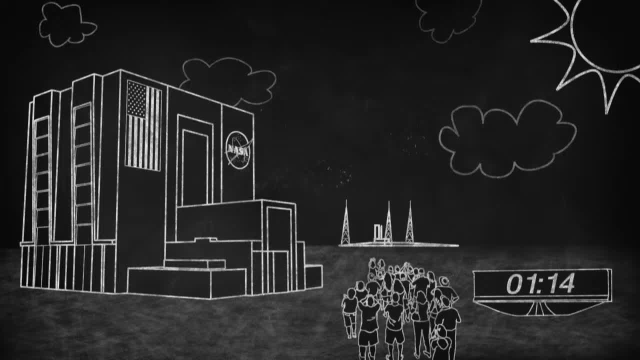 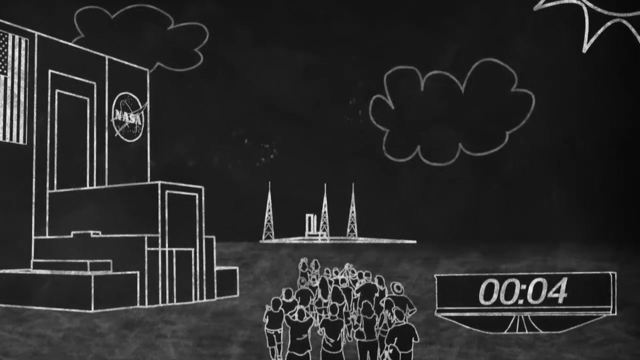 T-minus one minute, T-minus 30 seconds. We are go for launch. T-minus 10, 9,, 8, 7, 6, 5,, 4,, 3, 2, 1.. Welcome to the NASA social. 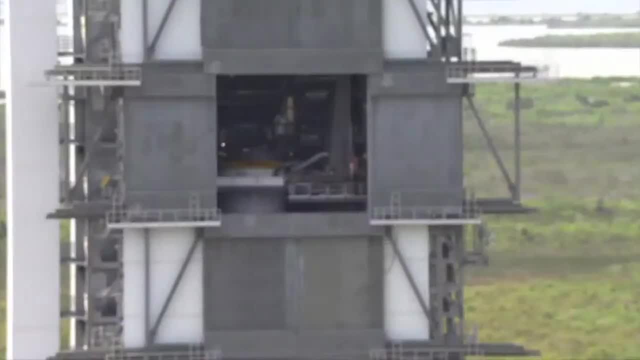 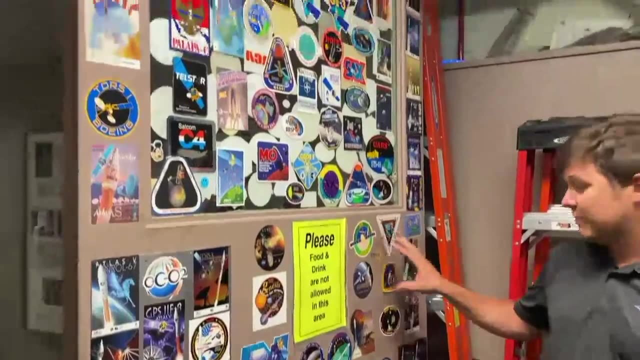 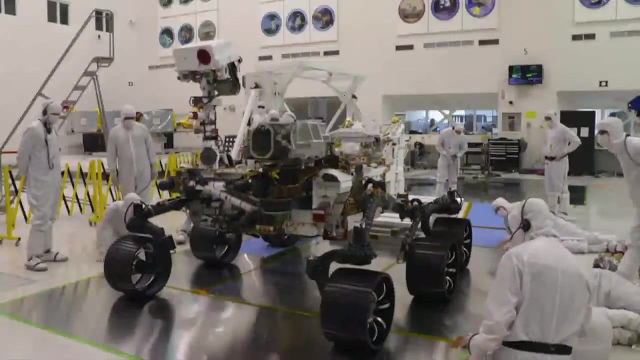 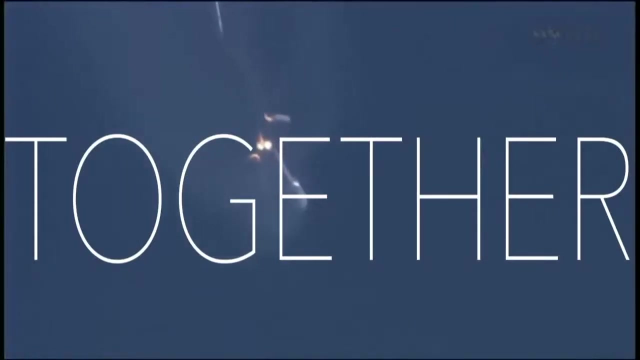 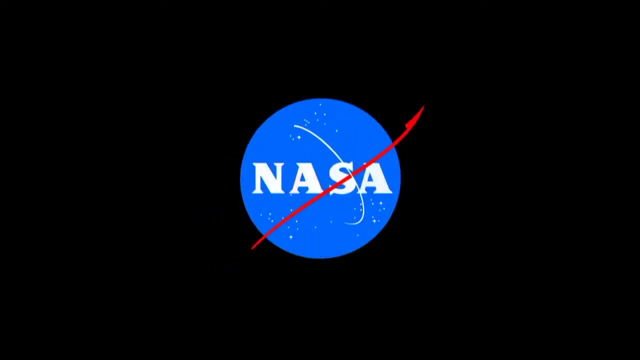 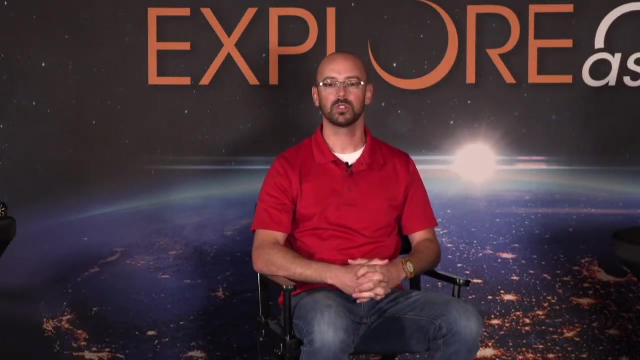 Welcome to the NASA social. Welcome back to the NASA virtual social for Mars 2020.. I am your host, Wayne Saxer, And on this episode, the final one, we are going to be talking about nuclear batteries. Joining me is my co-host, Allison. 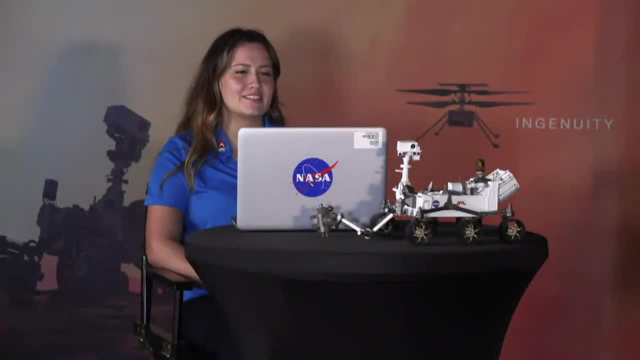 Allison, how are you doing today? I'm doing great Wayne and I'm so happy to be your co-host today And for everyone who is joining us live. I've been monitoring your questions for the earlier shows. I think you guys are going to be really excited about the guests. 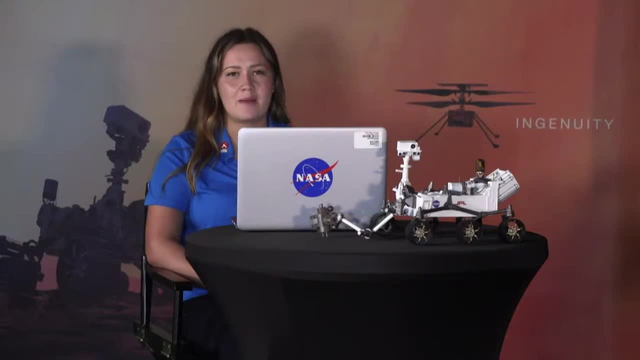 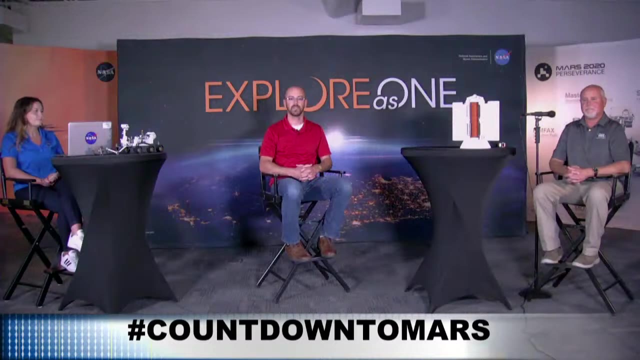 We have with us today. So please drop your questions in the comment box- Hashtag countdown to Mars- And we'll see if we can get most of those questions answered for you. Yeah, as Allison said, we have a great show prepared for you. 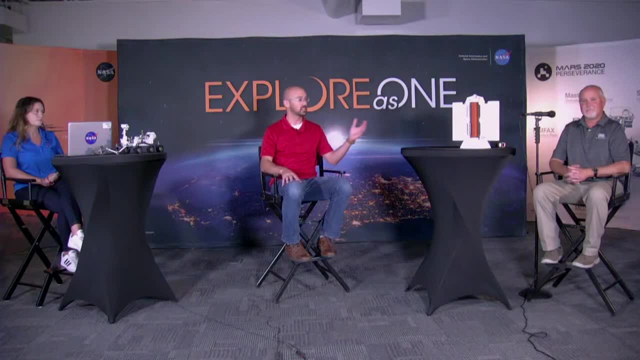 Like I said, talking about nuclear batteries, We have a guest joining us. We will introduce him after this video And we want to show you what does it mean to persevere. How did this rover get its name? We, as a species and as a company at NASA, we want to know. 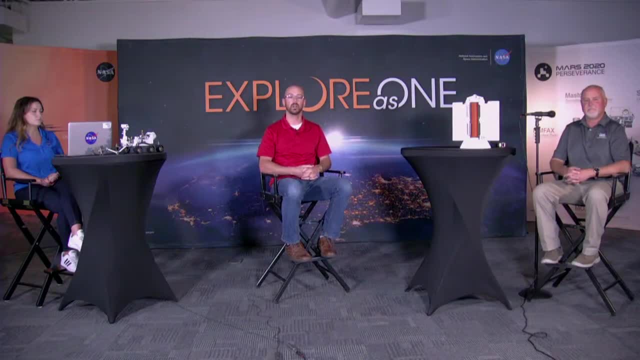 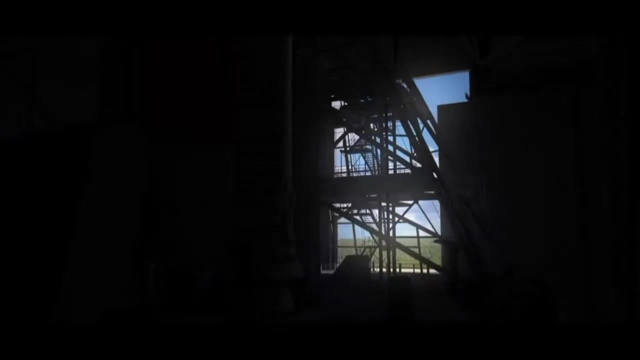 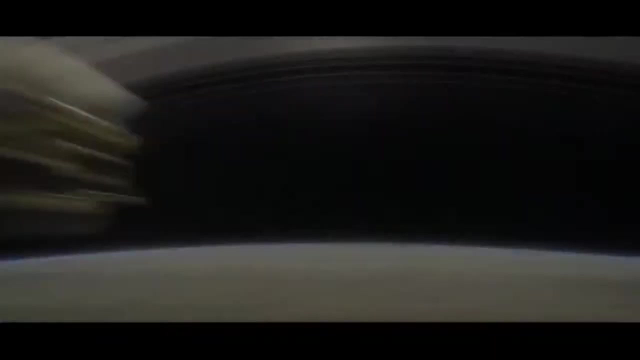 What it means. So please take a look at this video and we will come right back. We are a species of explorers- Believers. We choose to go to the moon in this decade and do the other thing, Not because they are easy, but because they are hard. 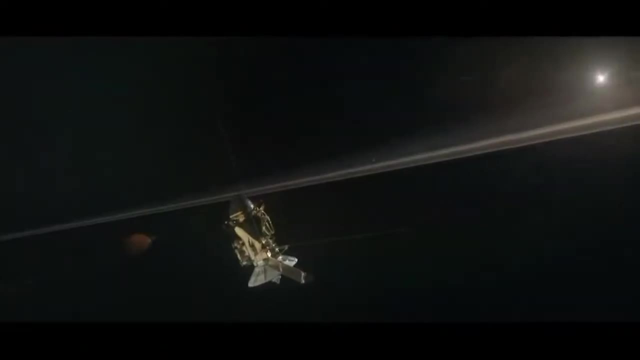 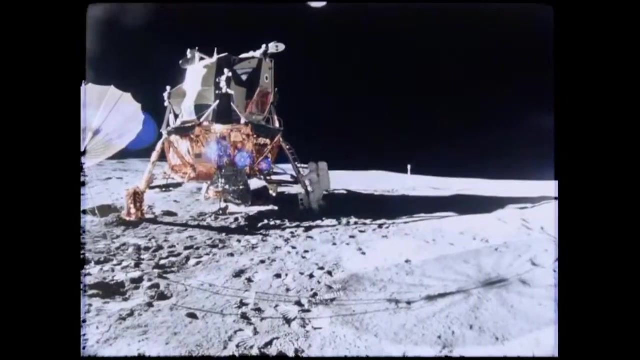 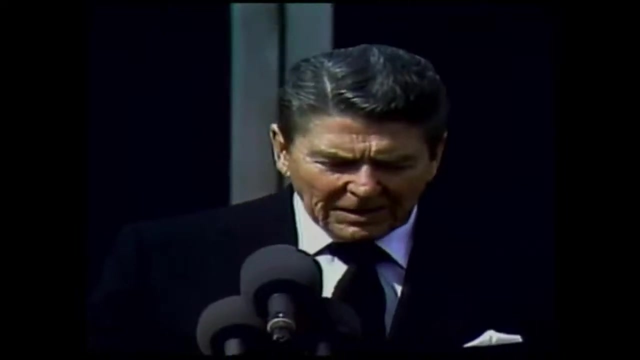 We are willing to do the hard things, to overcome the many challenges. This is what brings out the best in us. We are go for a mission to the moon. Our path has led to success And to bitter losses. We come together today to mourn the loss of seven brave Americans. 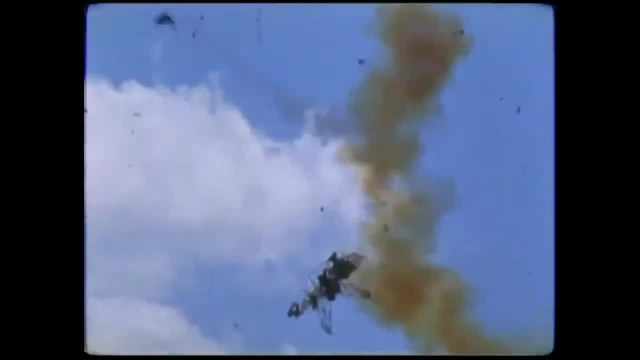 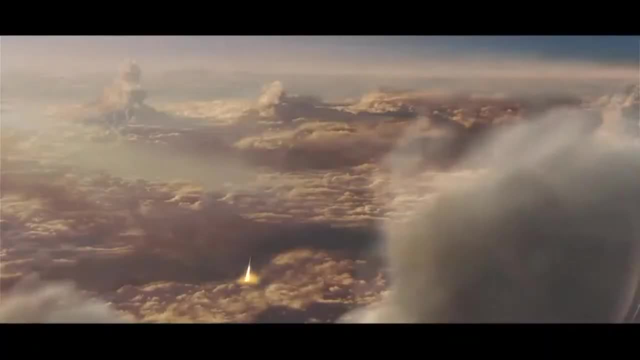 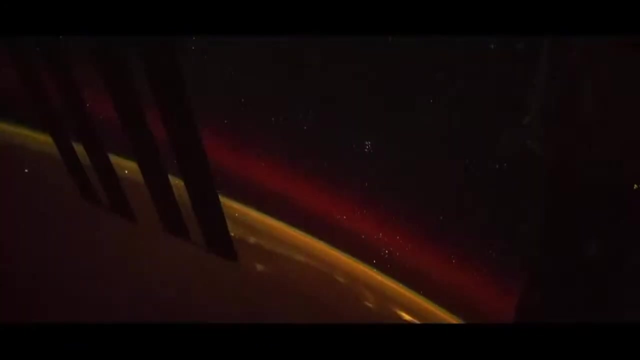 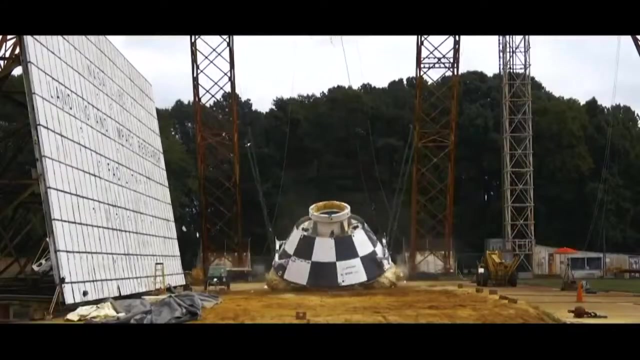 Yet, even when faced with tragedy and setbacks, we persevere, We keep striving, We keep believing. From space we see our planet as a whole. We see the challenges facing it And we face those challenges together. We will not give up. 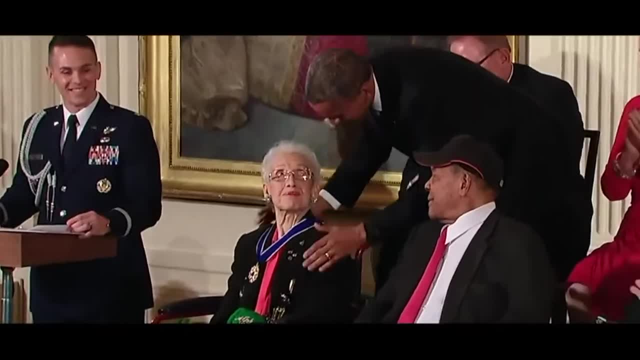 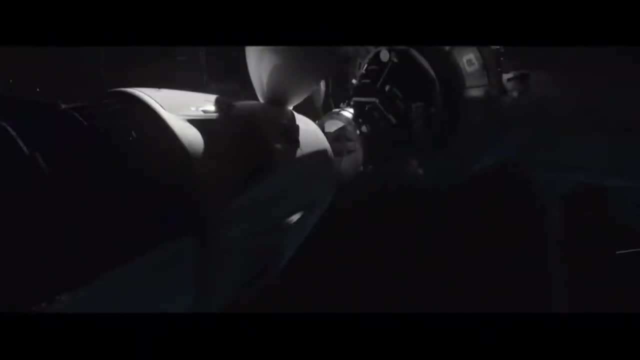 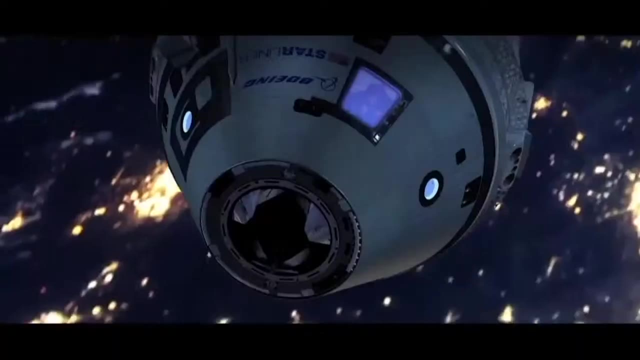 We challenge convention, We refuse to accept the status quo. The time at hand is hard, But we will persevere. We can still draw hope from the moon and the stars, From space, From exploration. There is a new day beyond the challenges we face now. 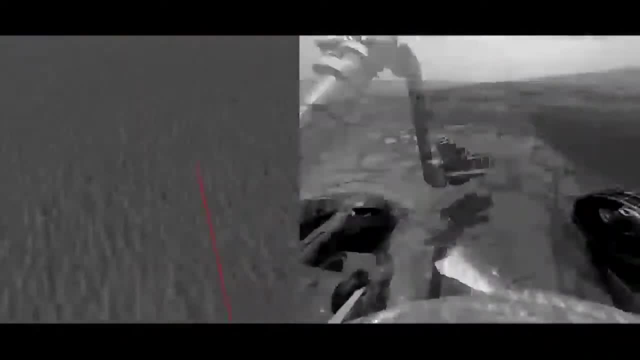 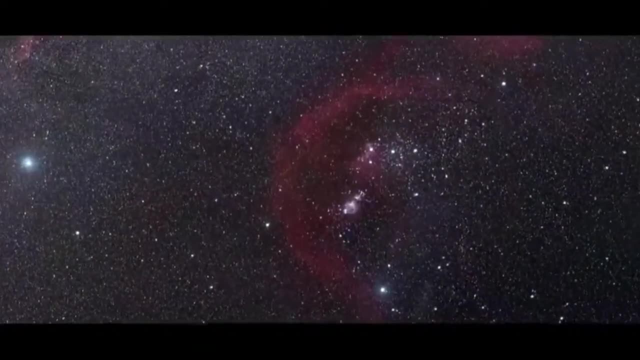 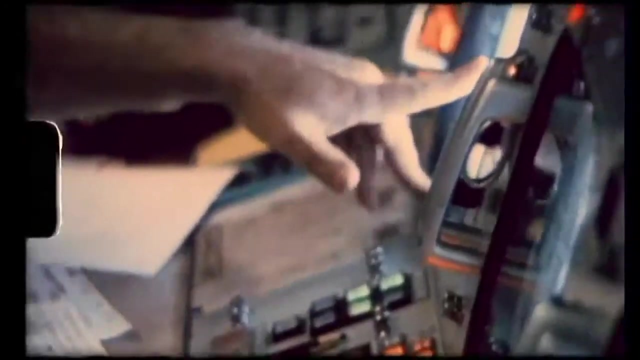 Curiosity, Insight, Spirit Opportunity. If you think about it, all of these names of past Mars rovers are qualities we possess as humans. Ten, nine, we have ignition sequence, start, But if rovers are to be the qualities of us as a race, we miss the most important thing. 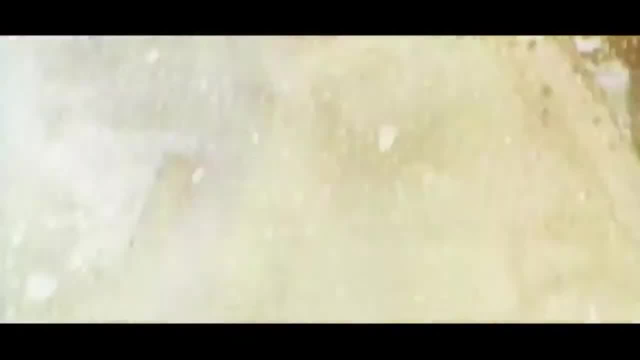 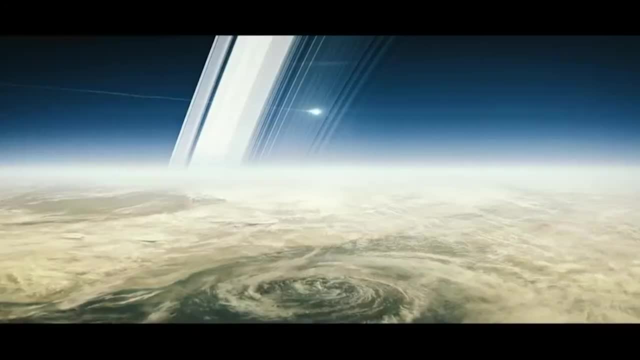 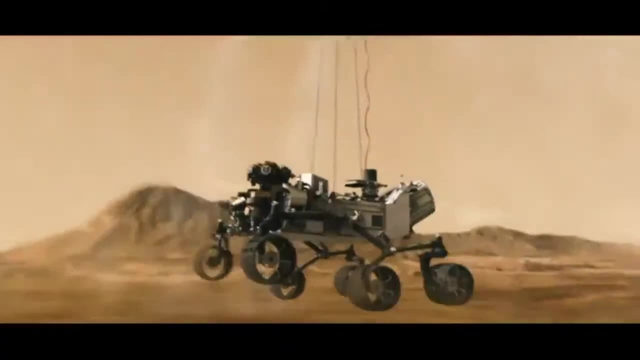 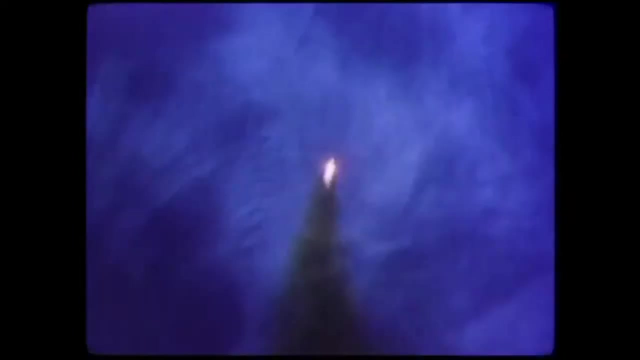 Three, two, Perseverance, Launch, commit, Liftoff. We have liftoff. We are a species of explorers. We are a species of explorers. We will meet many obstacles on our way to Mars, But, as humans, we will not give up. 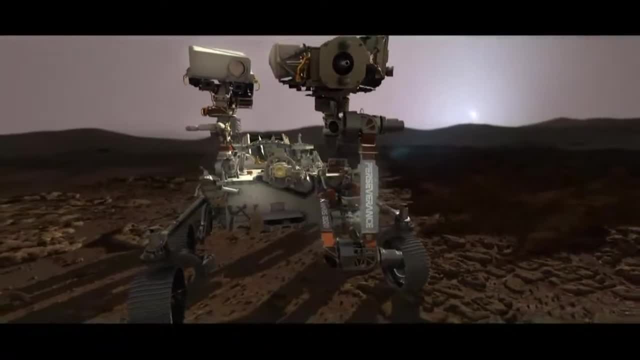 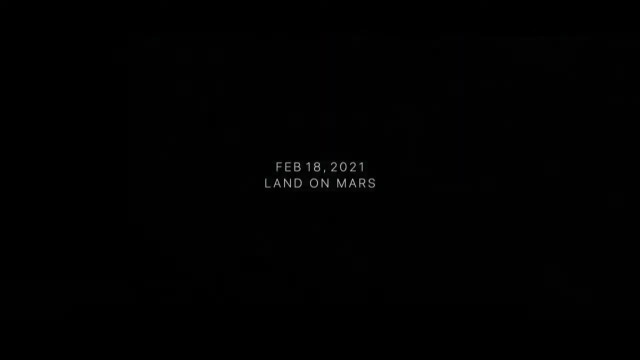 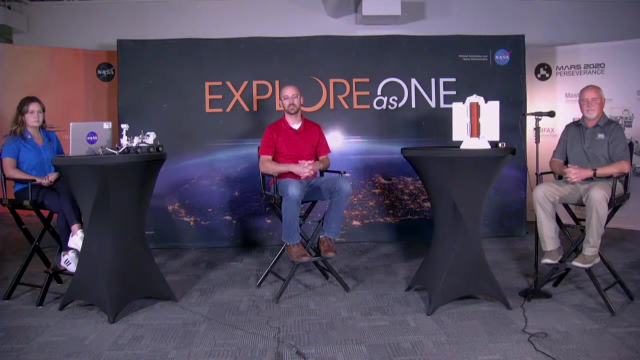 We will always persevere. As you saw there, the name perseverance definitely made it into the graphics. perseverance definitely has meaning to us. And speaking of names, it's not just called a nuclear battery, It's a multi-mission radioisotope thermoelectric generator. And here to talk to. 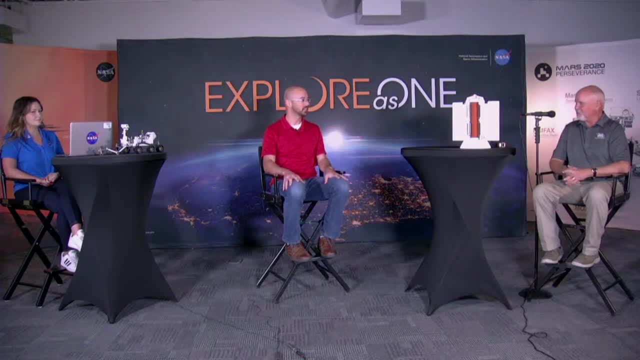 us about it is Greg Hula. Greg, how are you doing today? I'm doing well, Wayne. Thank you, You're welcome. Can you tell us a little bit about what it is and on what the MMRTG is? what your role? 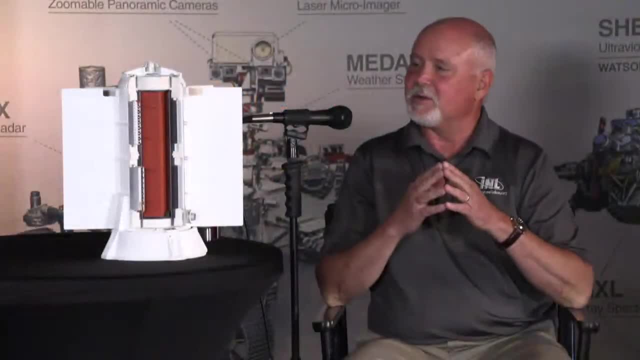 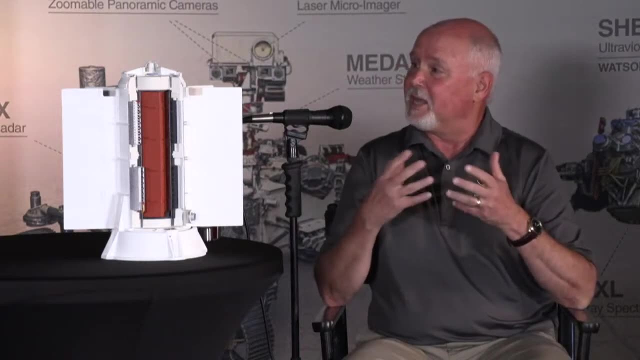 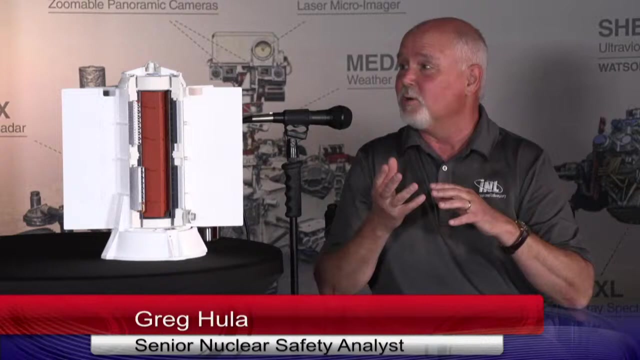 with it is and kind of what it is you do. Yeah, So the MMRTG, as Wayne mentioned, is a nuclear battery. It's essentially a system that converts heat from the natural decay of radioisotope fuel into electrical power, And that's power that will provide electrical power for the rover. 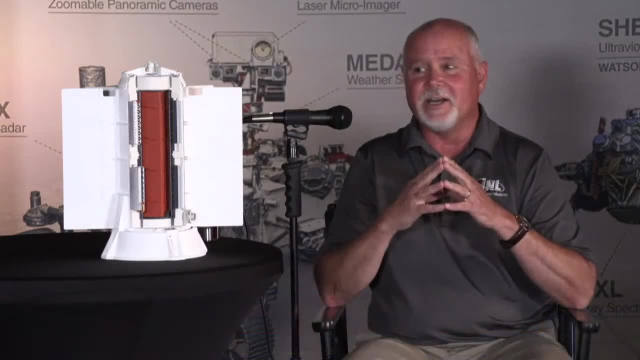 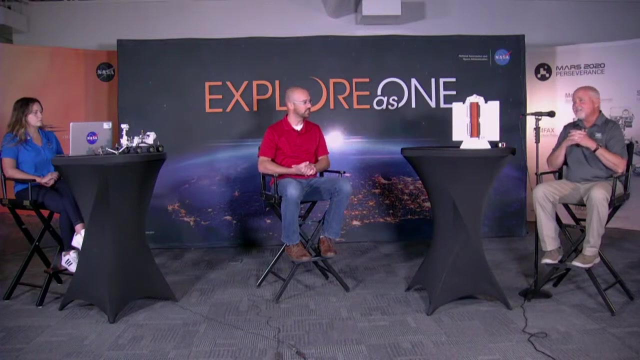 on the surface of Mars. Our role at the INL for the Mars 2020 mission includes the assembly and the testing and the delivery of the power system for the rover. You said INL. Can you tell us what that is and what your role there is? 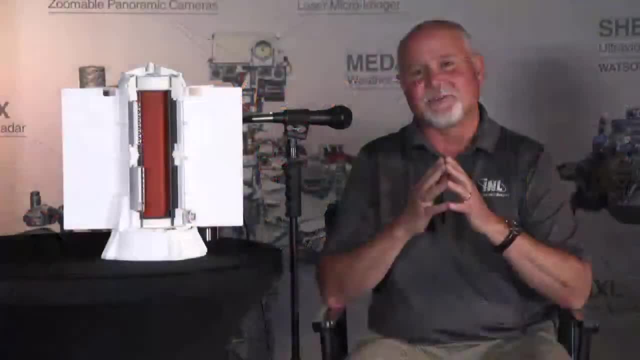 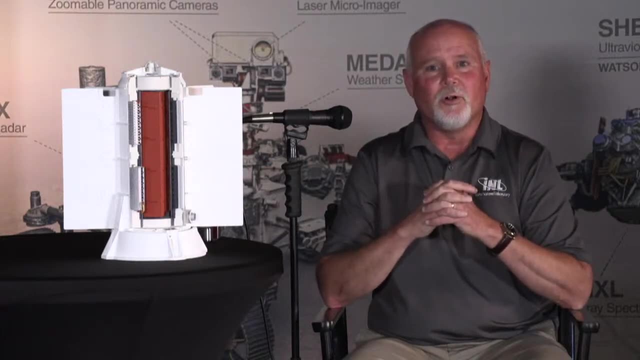 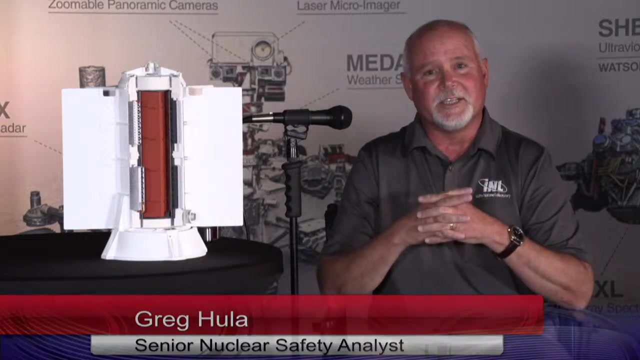 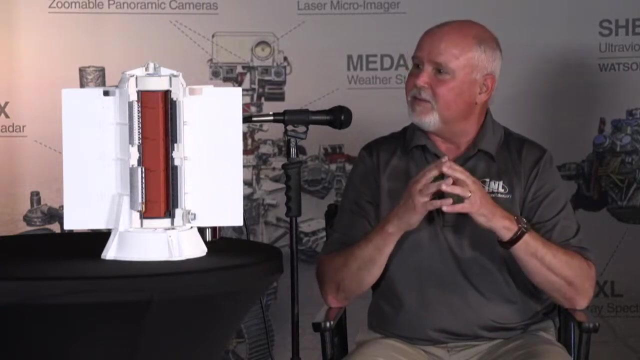 Yeah, I can. INL stands for Idaho National Laboratory. We are part of the Department of Energy's complex And our role at the INL in the Space Nuclear Power Division, which is the group I work in, my role in that division, is nuclear safety And we look at the safety of the RTG. 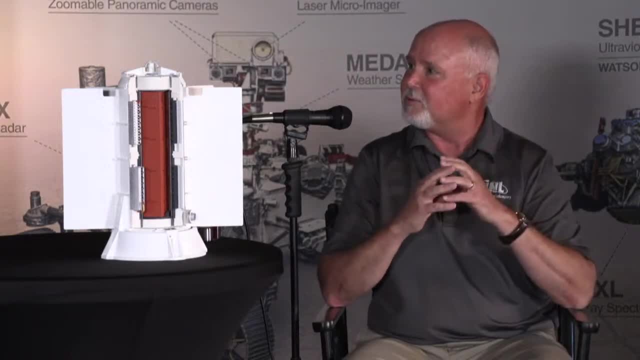 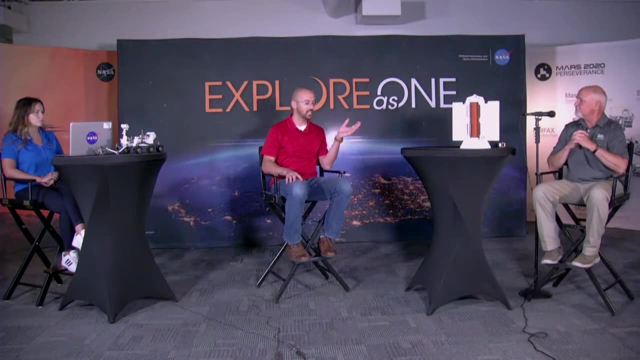 power system in context of facility operations, transportation and, most recently, in some launch safety context, Wow. So I spent some time researching this and I could ask you tons of questions, but this is all about our viewers, So we're going to jump right to Allison. Do we have any questions coming in from social 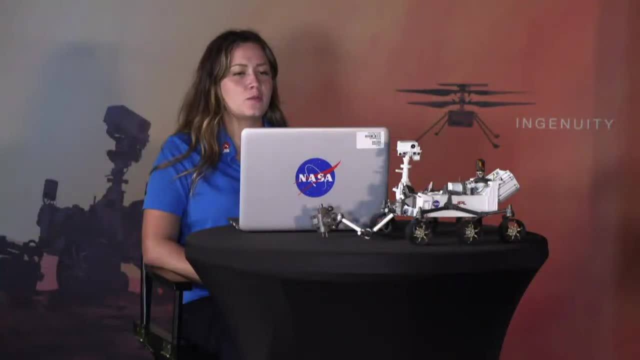 Yeah, our viewers are definitely excited to learn about this. First, can we talk about a little bit the difference between switching from the solar panels to this nuclear battery and what the pros of it are. Yeah, there's a couple of benefits of using a system such as an. 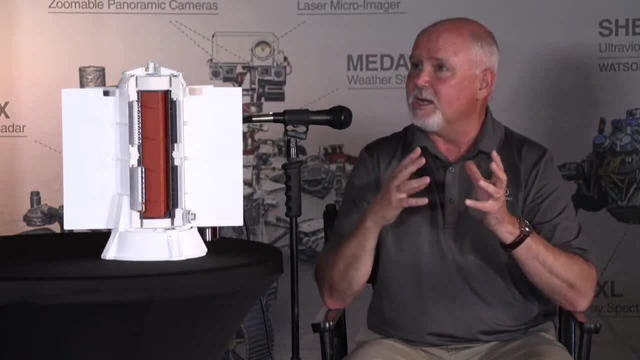 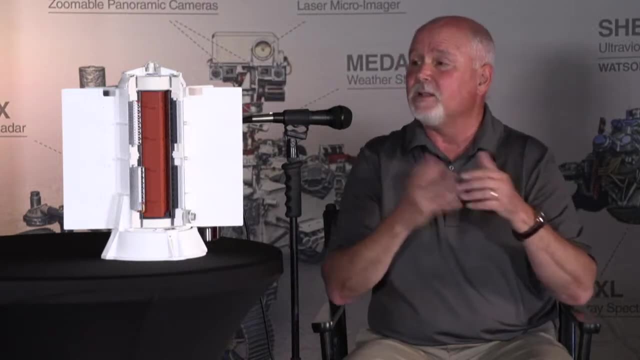 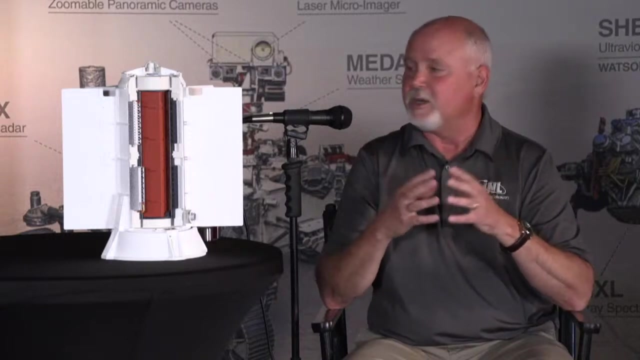 RTG. One is the RTG is not affected by, say, dust that might accumulate on a solar panel and reduce the efficiency of the panel. The RTG is a completely sealed system So you don't have impacts of dust or their planetary environments that may degrade adversely affect the system. The other benefit is 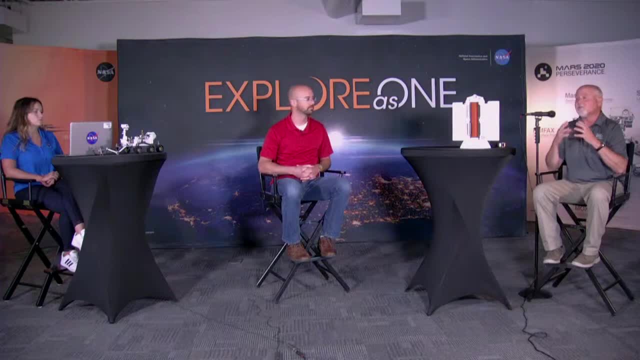 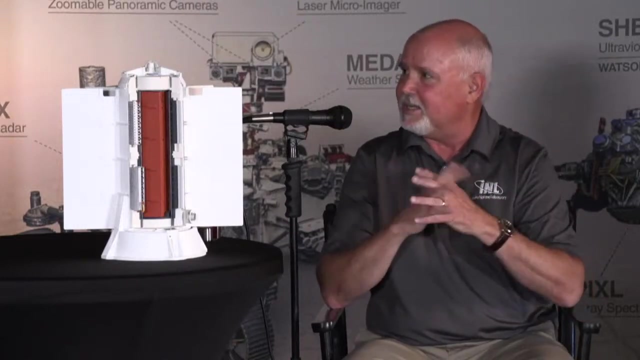 that the nuclear battery provides power 24 hours a day over the course of many, many years And the It doesn't have adverse effect from, you know, sun not shining, et cetera, evenings, days, nights, days, nights. 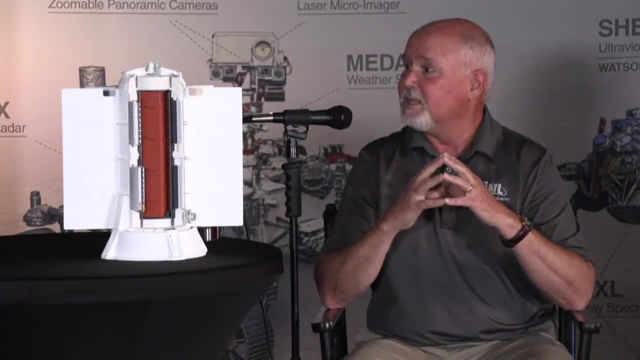 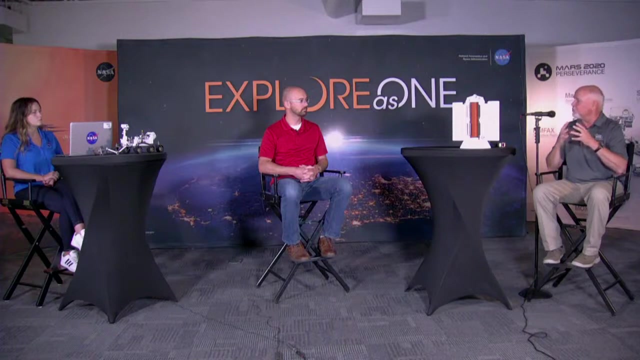 So it's a very reliable source of power and it's actually got a design life of about 17 years And we expect that source of power, the RTG, to provide power for as long as the mission and the rover need it. 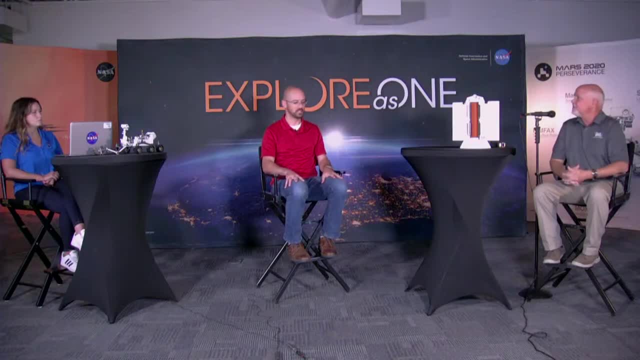 Yeah, that's really cool. I was talking to my brother last night and that was his first question is well, if we're not using solar panels, then you know how long is this battery going to last? So to hear it's going to go 17 years, like that's a pretty long life cycle, for you know something that's being sent to another planetary body. 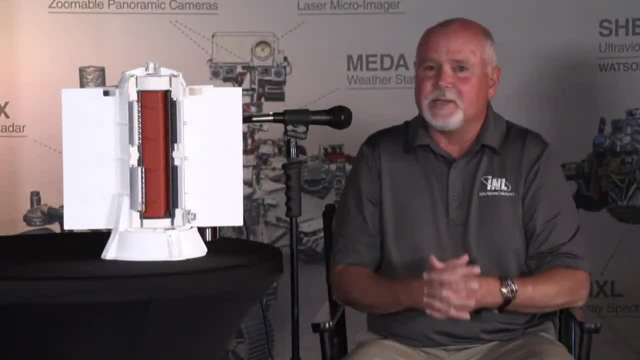 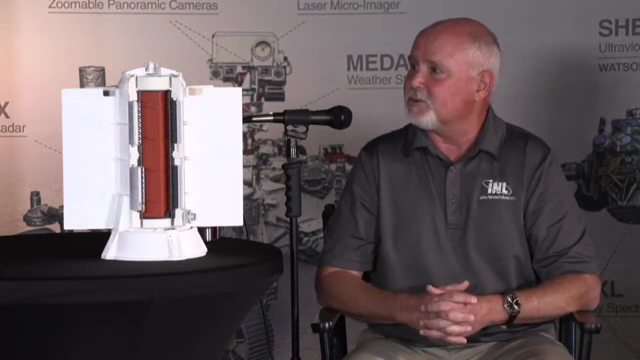 It is, And these RTGs have been used by NASA, provided by the Department of Energy, for over 50 years, going back to the late 60s, early 70s. They've been reliably used as sources of power, Not only for solar power. 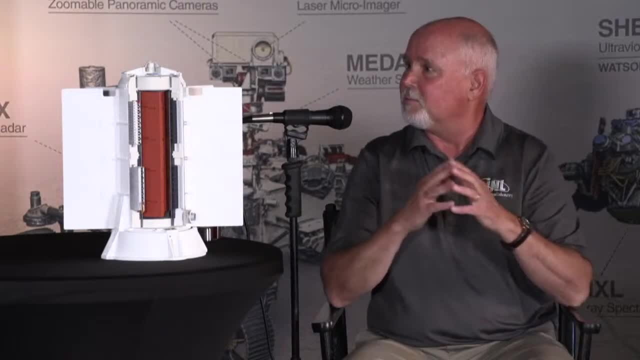 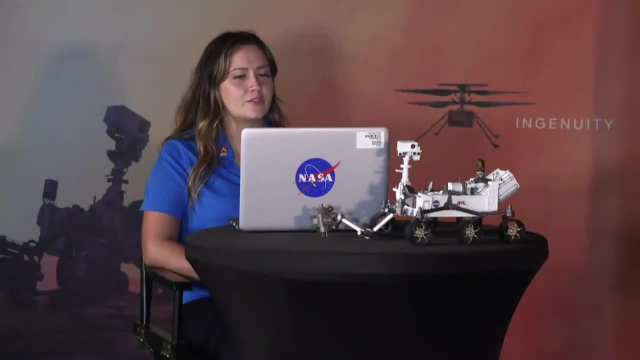 Not only for deep space missions, but also for missions such as the planetary surface on Mars. Yeah, Wow, Allison. do we have another question coming in from social? Yes, we do So. our viewers want to know: is this the only power source on the Perseverance rover? 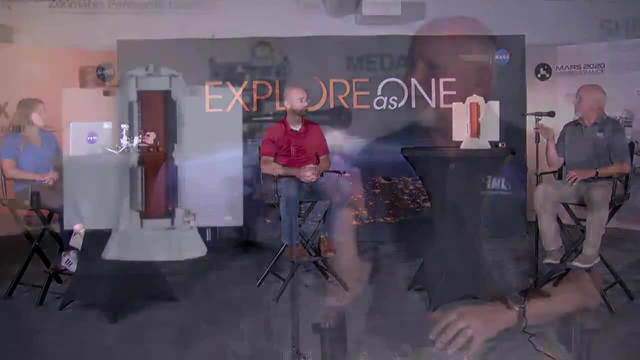 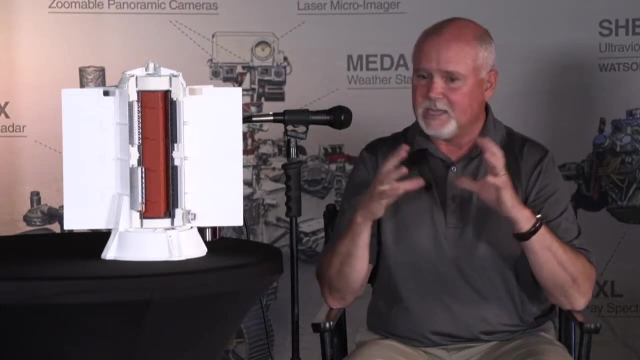 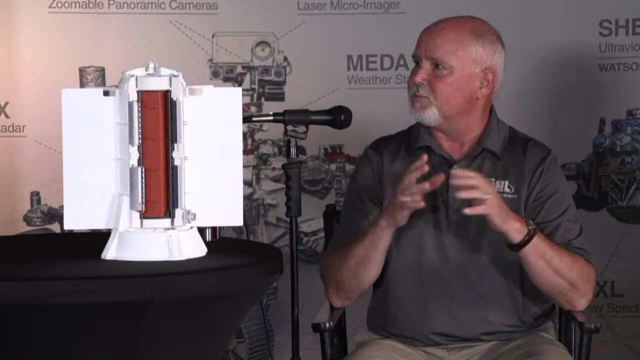 This is not. This RTG provides power to lithium ion batteries And the lithium ion batteries can store up the power provided by the RTG and meet peak demands, And meet peak demands of the Perseverance rover's instruments and scientific packages. 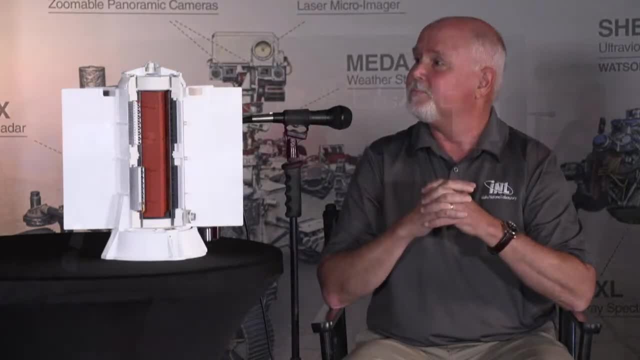 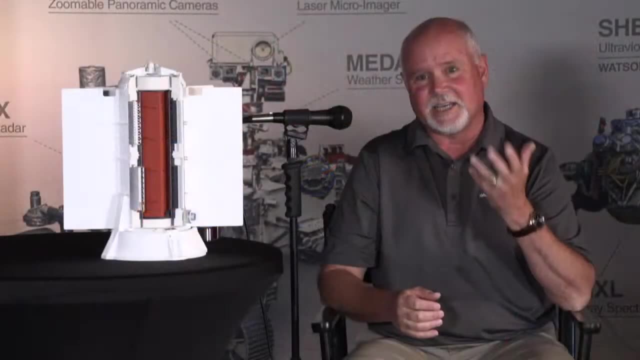 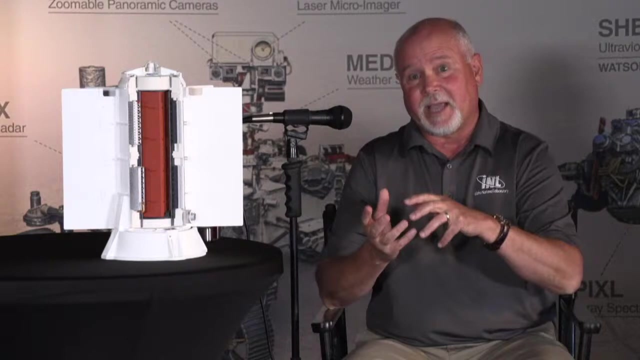 It is the only nuclear power system on the rover, though. Awesome. And then what's next for the MMRTG? Well, the MMRTG was successfully integrated to the rover last week. We mean integrated in the sense of attached electrically and mechanically. 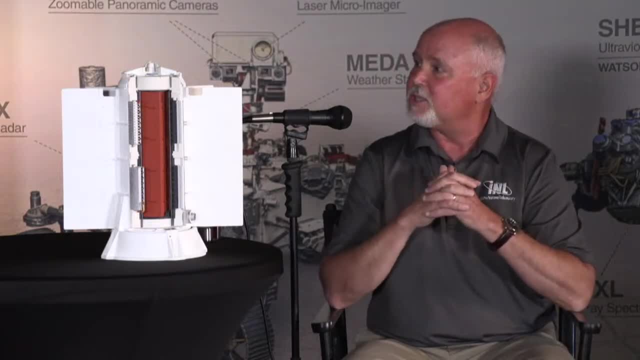 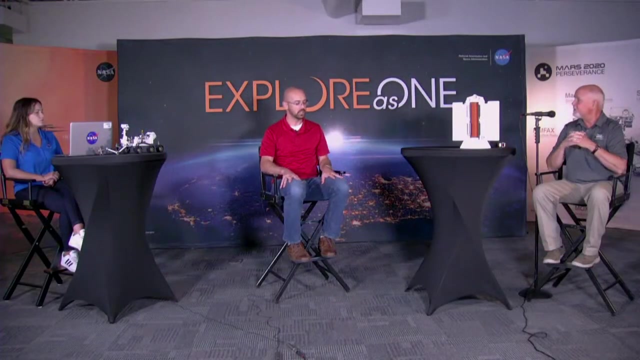 And with the Perseverance rover we launched successfully tomorrow, And once on the surface of Mars, the RTG will provide power to the rover for many years. And so I actually have this question. We get this a lot. Can you talk a little bit? when you hear nuclear battery, I think that makes people a little nervous. 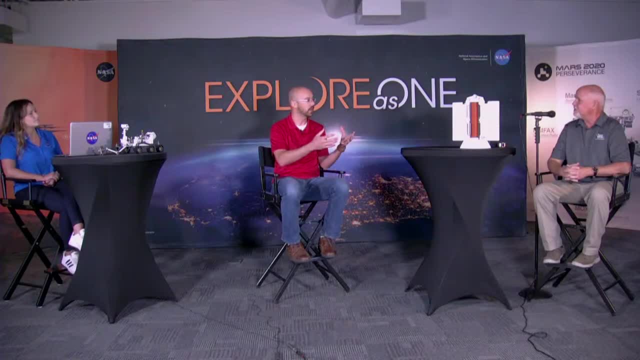 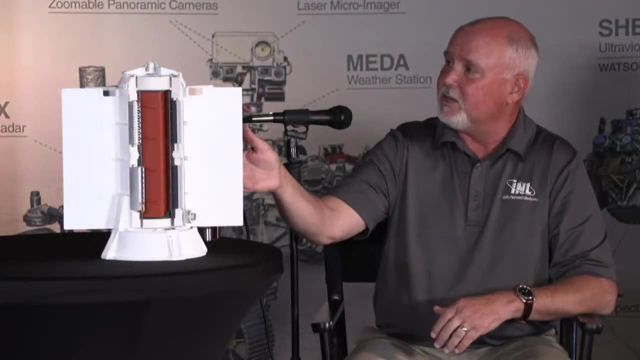 Sure, So can you talk about kind of what it means for it to be a nuclear battery and some of the safety that's been implemented? Yeah, I can We have a kind of a half-size replica of the RTG, the multi-mission RTG? 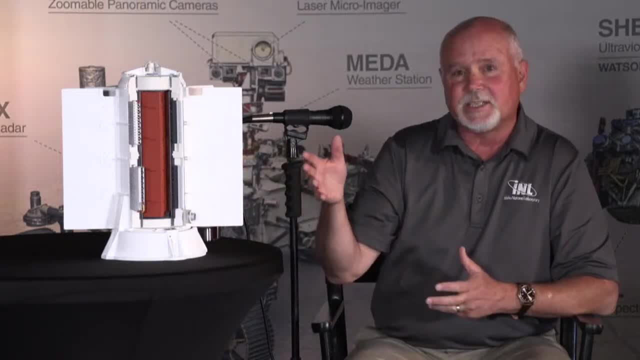 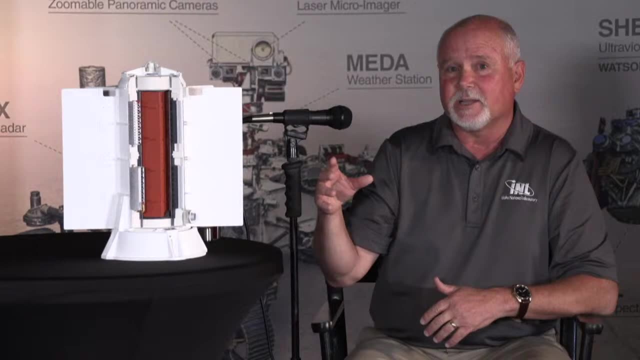 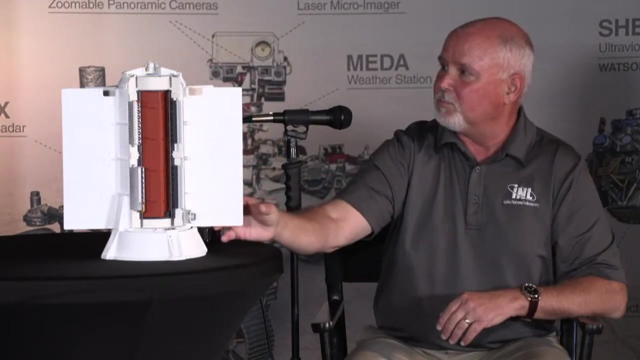 Okay, And, as I mentioned, it's a system that converts the heat from the natural decay of radioactive material to electrical power, And it essentially consists of two parts At the center of the unit, as shown in the orange blocks. that's the heat source. And the heat source consists of about 10.6 pounds of plutonium dioxide fuel And the main isotope in that fuel that produces heat is plutonium-2-3.. That heat source is surrounded by 768 thermocouples, the thermal converter part of the system. 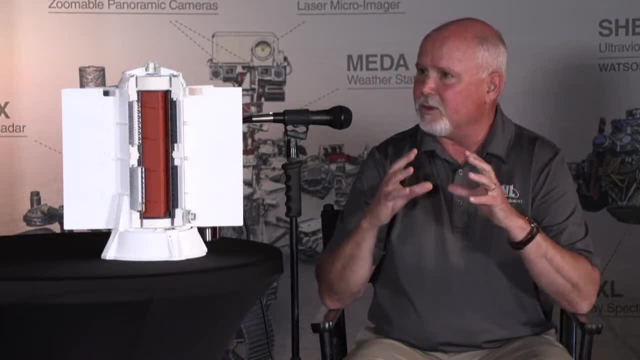 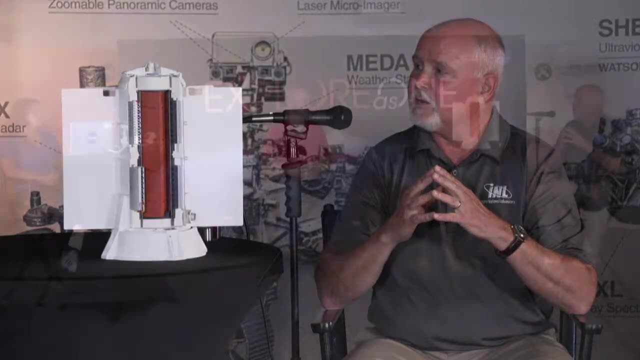 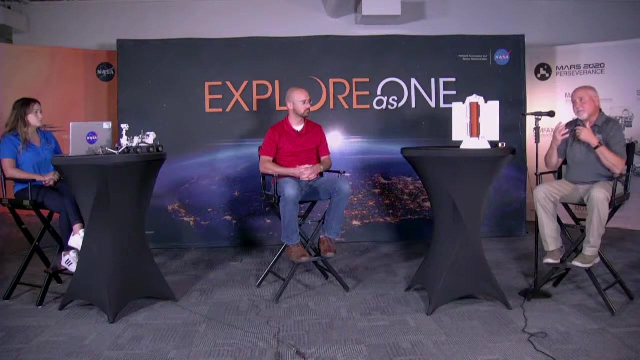 And those thermocouples are collected, They're assembled into an electrical circuit that converts the 2,000 watts of heat into approximately 110 watts of electrical power for the rover And the ability to use a system like this a nuclear power system. 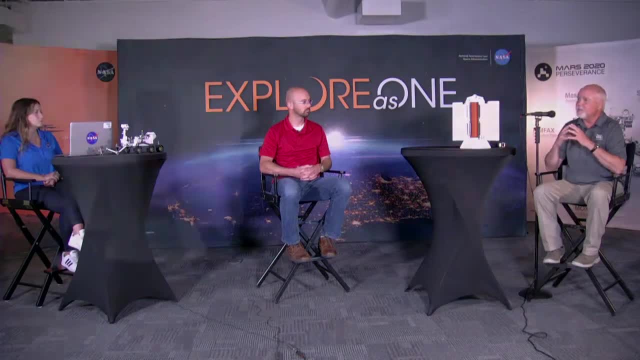 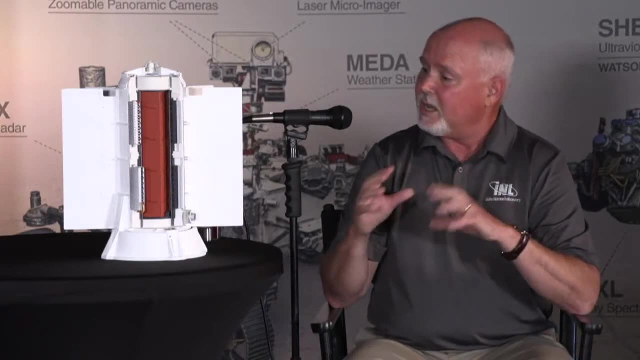 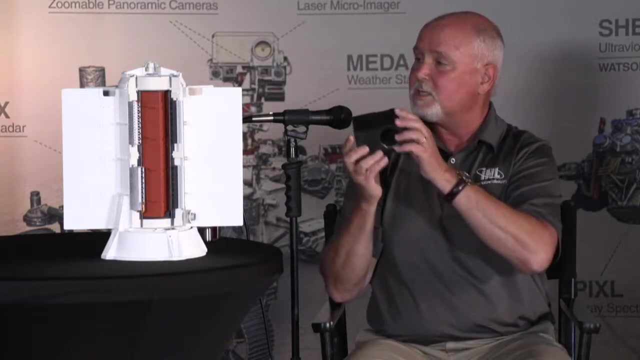 such as an RTG is largely possible because of the very high degree of safety that goes into the heat source, And by heat source I mean the blocks. They're called general-purpose heat source modules And it's about 4-inch by 4-inch by 2-inch block. 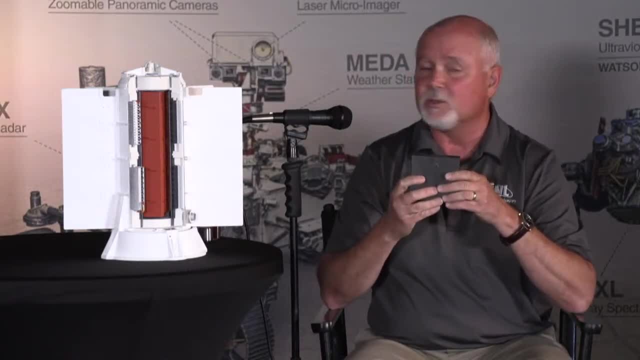 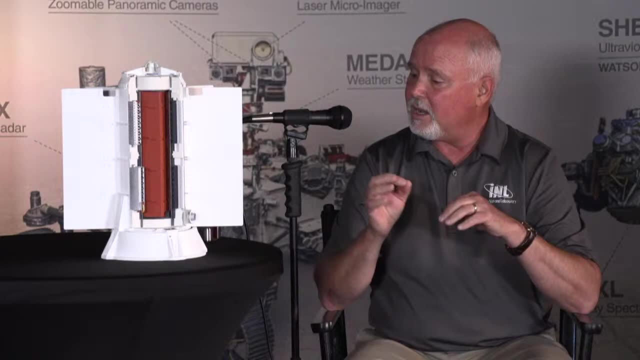 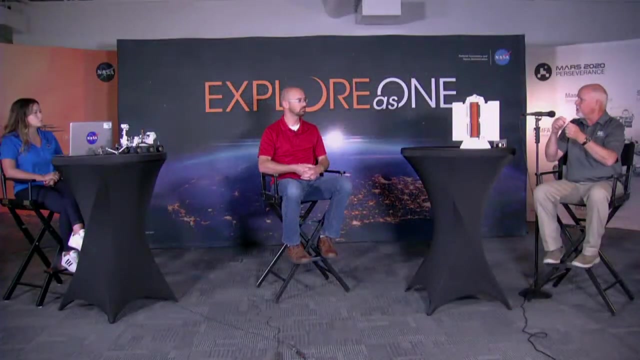 And these are the heat sources that contain the plutonium oxide fuel. And the general-purpose heat source is composed of several parts And I'm going to talk or describe it from the inside out. And if you think about an onion, if you were to peel the layers of an onion back until you got to the inside, 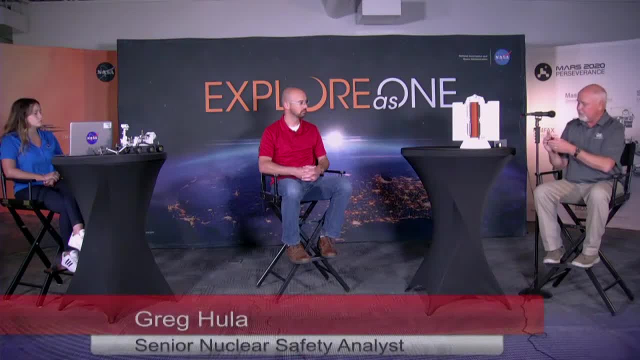 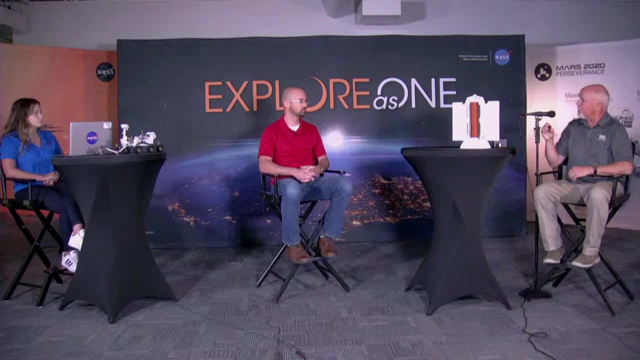 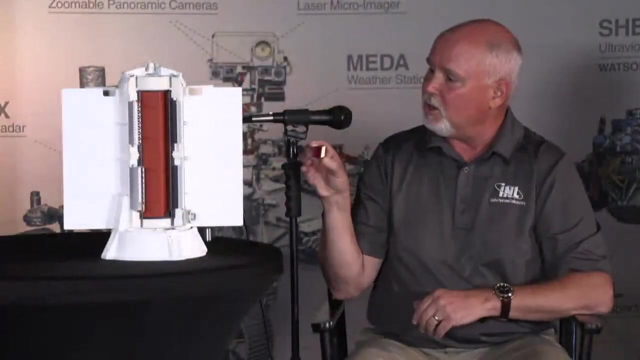 we'll start at the inside of the general-purpose heat source And at the inside is the fuel. I've got kind of a model of a fuel pellet here And the red reflects the heat generated by the plutonium-2-3.. This pellet's about 1-inch tall and about 1-inch in diameter. 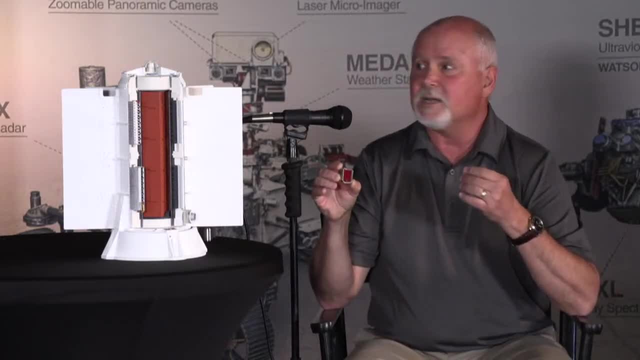 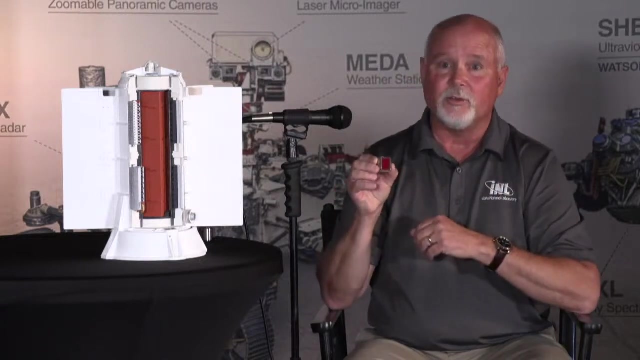 That fuel is a ceramic form of plutonium dioxide, And the benefit of ceramic is that under impact accident environments it will tend to fracture or break into pieces and particles that are largely too large to be carried away by wind. The containment of that fuel, pellet, is provided by an alloy of iridium called DOPE-26.. 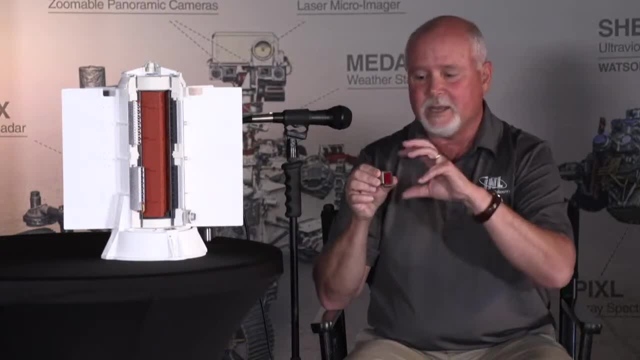 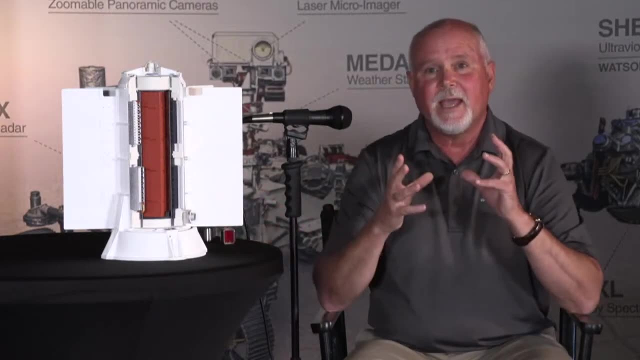 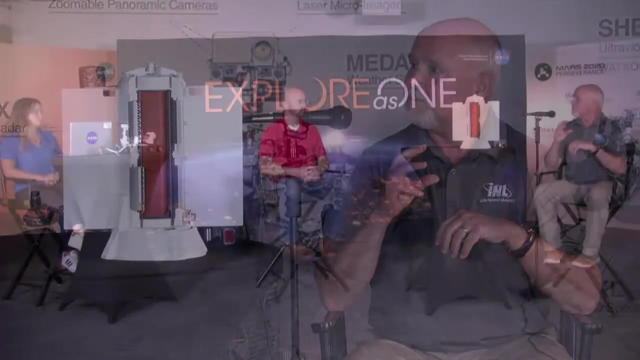 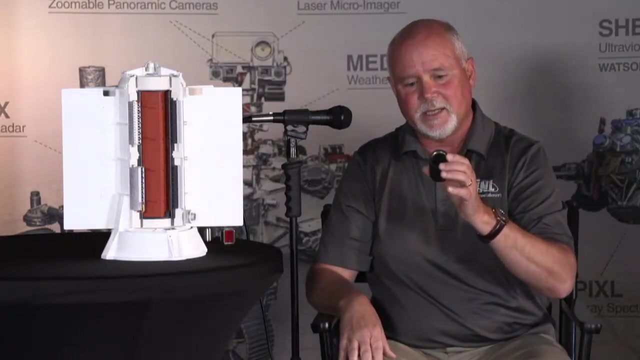 And that It's basically a metal casing that encapsulates the plutonium oxide pellet and provides for the containment of the fuel. Surrounding that fuel clad are three very special layers of carbon material. The first one is called a graphite impact shell And it's a cylindrical component. 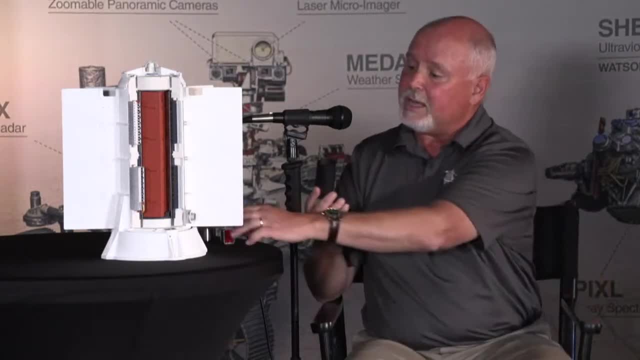 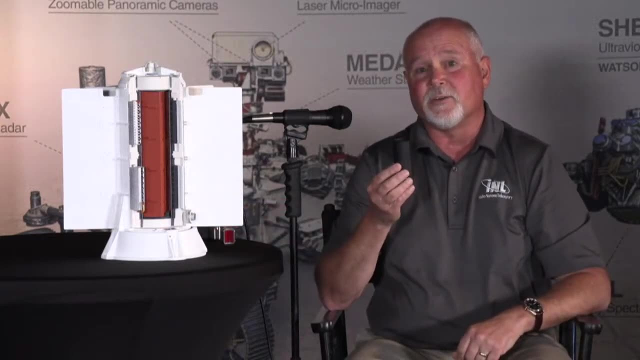 It's about 2-1⁄2 inches long and it holds two of the fuel clads. The fuel clads would sit inside of the graphite impact shell. This graphite impact shell provides protection under very energetic impact scenarios. And are these to scale? 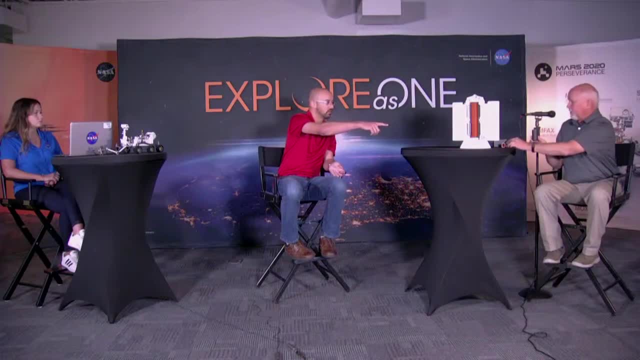 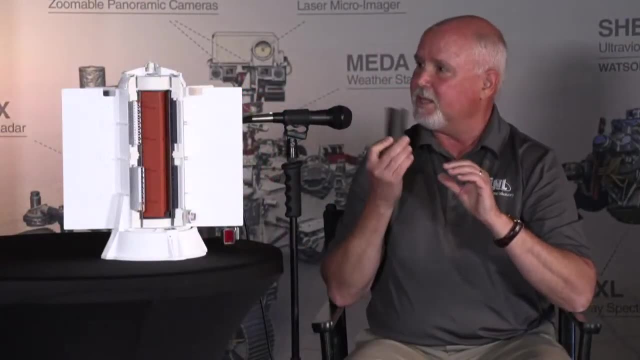 These are to scale And we have a hat scale model here. right, That's correct, But these are to scale. Yes, The components that I've got for the GPHS module are to scale, Cool. And then surrounding the graphite impact shell is a carbon-based component. 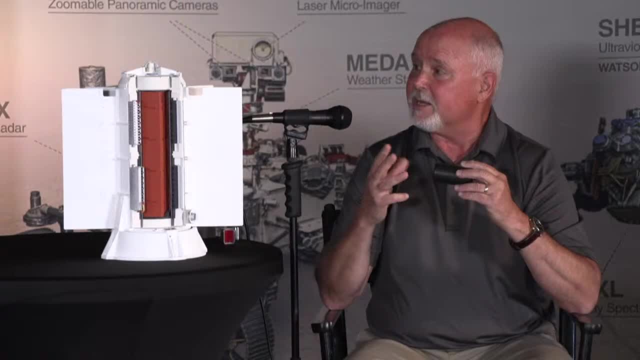 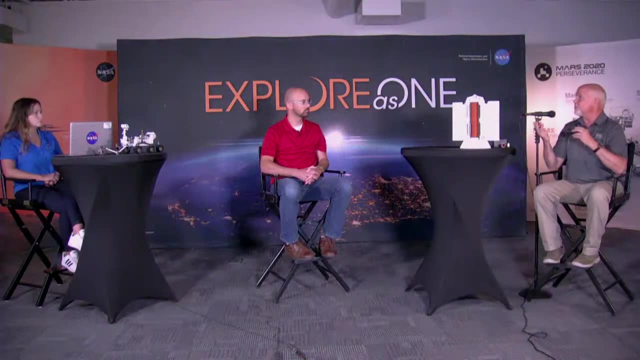 that basically serves as a thermal insulator. So under the very high-temperature environments associated with atmospheric reentry, that thermal insulator serves to protect the fuel clad from extreme temperatures associated with atmospheric reentry. So it sounds like what you're saying is. 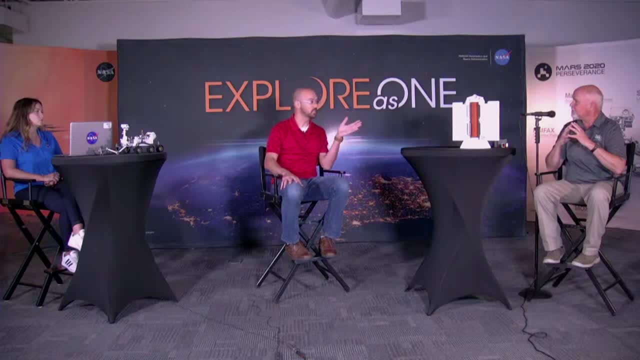 in the extremely unlikely event of a contingency, that this will actually protect the plutonium. what you said on reentry, So this can survive a reentry all on its own. It is designed to survive a reentry, That's correct. 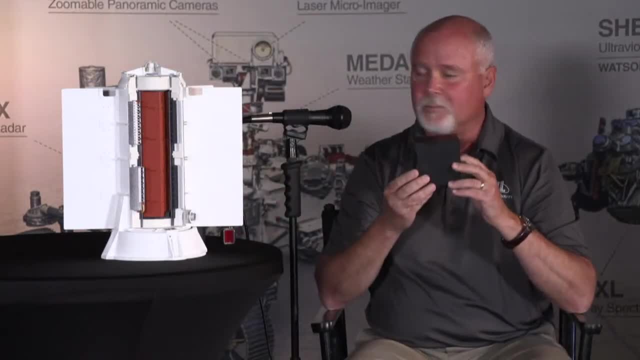 Okay, The outer, most protective layer, which is the most substantial part of the GPHS module, is what we call the aeroshell, And the aeroshell is designed to accommodate two of the graphite impact shells, such that there's four fuel clads in each GPHS module. 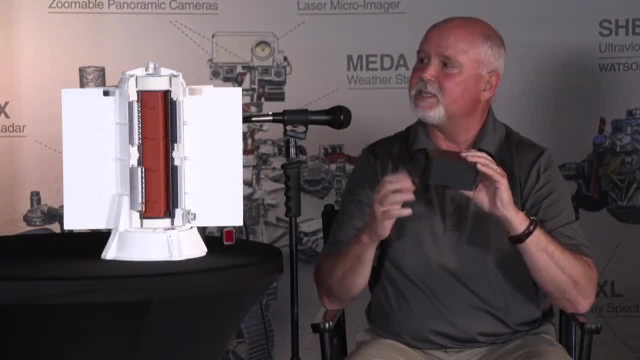 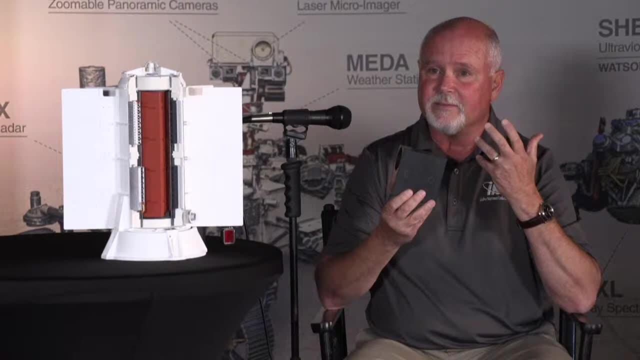 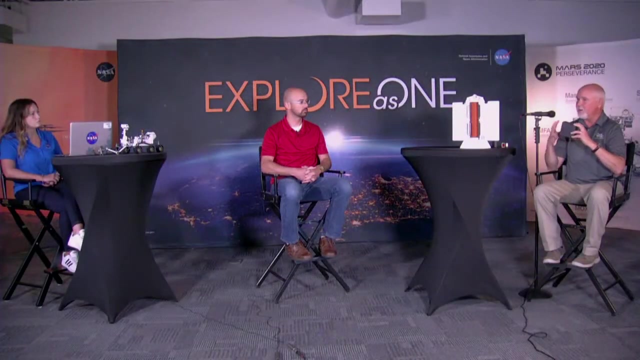 This aeroshell is made of the same material, similar material that's on the nose cone of a missile, So it's very, very rugged, very durable and provides a very high level of protection under impact as well as thermal environments. The components, when assembled into the aeroshell: 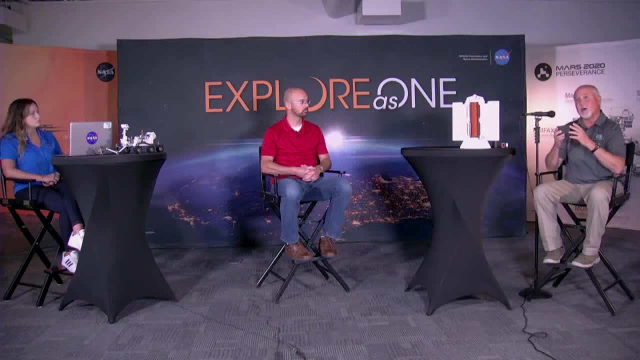 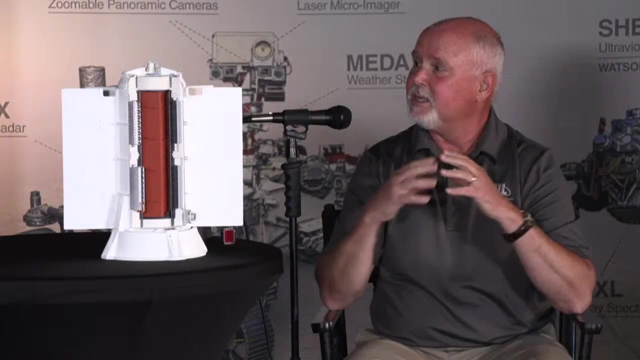 is what we call the GPHS or the General Purpose Heat Source Module, And there's eight of these modules that are stacked in the center of the multi-emission RTG and produce about 2,000 watts of heat from the plutonium-238 decay. 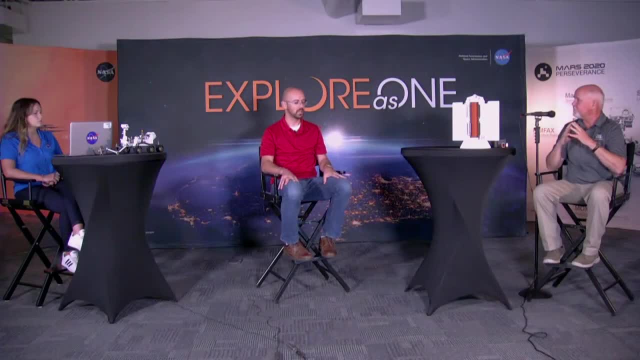 Wow, And so we were talking earlier, kind of behind the scenes, and I was told that you know, this is actually very, very safe. It's alpha rays, and the only thing that you need to not do is eat it. 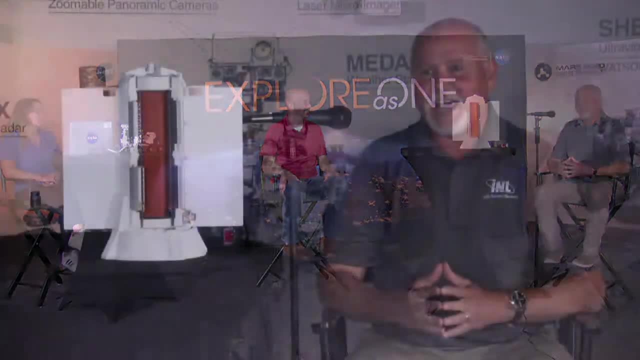 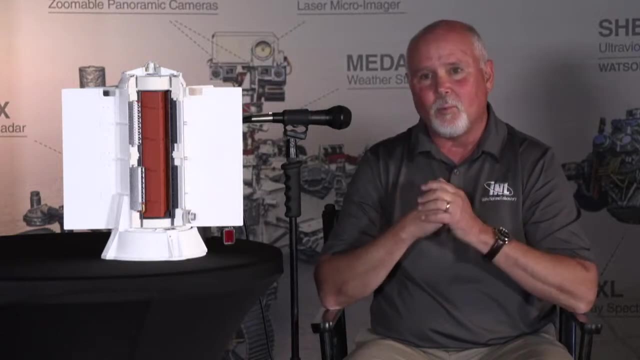 and that you would be fine, right? Yeah, You know actually, Wayne. what we don't want to do is have any of it released And eating. it is one way where it could get in the body. The other is through inhalation. Okay, So the General Purpose Heat Source Module is designed to provide a very high degree of protection for the fuel inside. It is possible under some very energetic accident environments There can be some small quantities of plutonium released And the concern with that, as you mentioned. 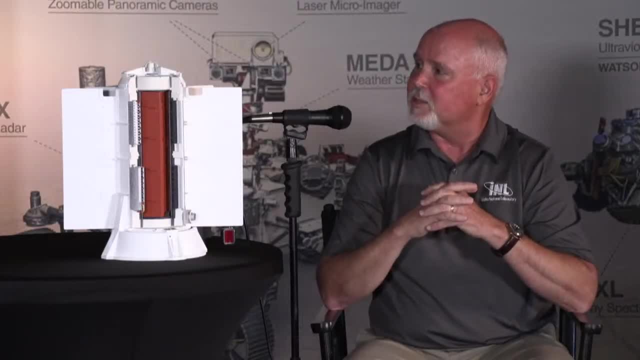 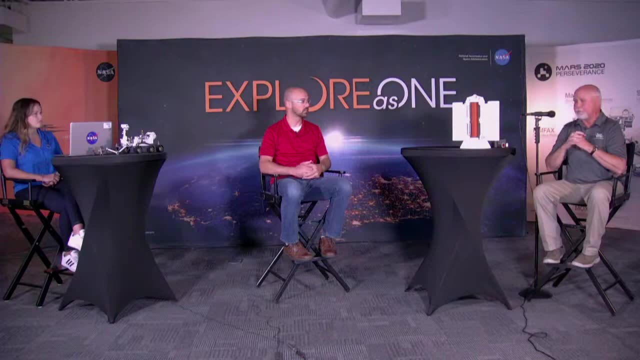 is the potential for health risk from those kinds of releases. But that's why we have these systems. we have backup systems and safety is one of our core values here, Absolutely, Absolutely. And we do have one last question from social: Why was the MMRTG attached at the very end? 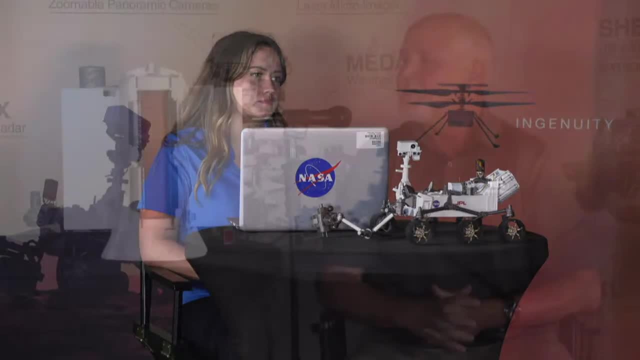 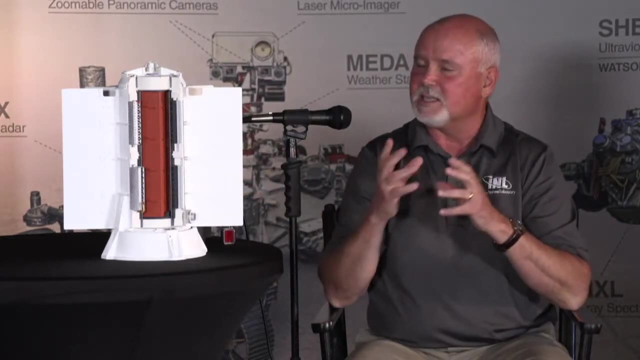 just before the rocket was about to roll out. So one of the reasons for that has to do with the fact that not only does the plutonium emit alpha radiation, but it also emits gamma and neutron radiation, which isn't easily blocked by the components. 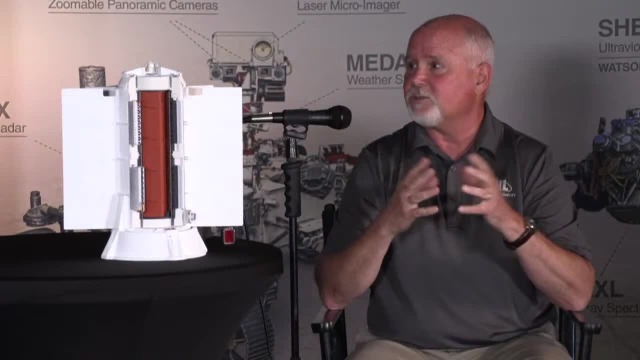 So that can be a health hazard to workers, a radiation hazard. It's not very big, It poses no health risk to the public. But by holding off on the integration of the RTG to the end or very close to launch, there's less people working around the RTG. 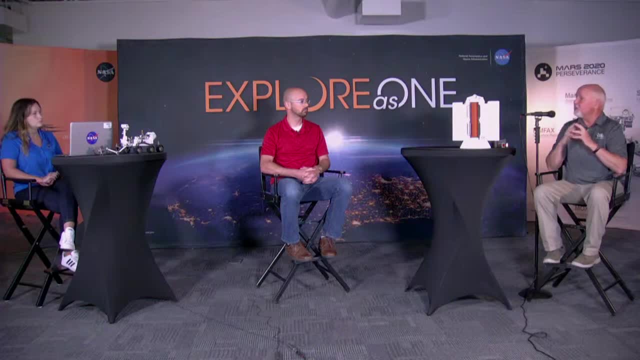 and exposed to that kind of radiation. And then also, I believe there's some serves to not introduce a thermal hazard early in the spacecraft assembly. So you're basically holding off on that, the heat that's generated or put off by the 238.. 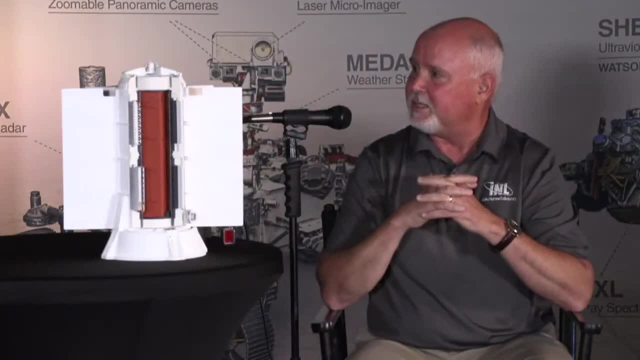 You don't have that thermal hazard present as well. That makes sense. So I got to say, after hearing you talk about this: I you know when you hear you're: oh, we're launching a nuclear battery on the Perseverance. 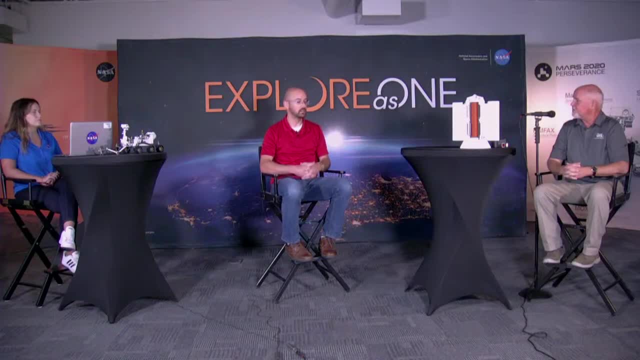 rover and sending it to Mars, like you do kind of feel a little uneasy, but hearing all the safety precautions that you know- INL and the Department of Defense, you know they've been talking about, oh, we're launching a nuclear battery on the Perseverance. 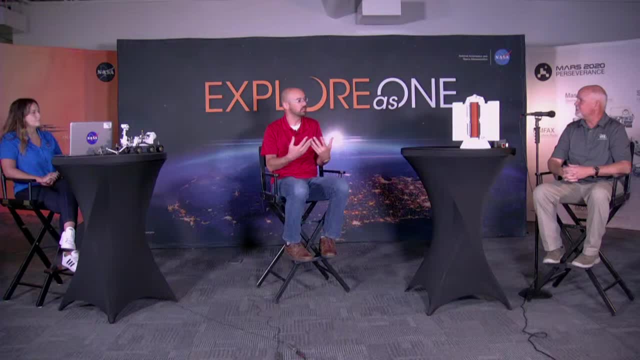 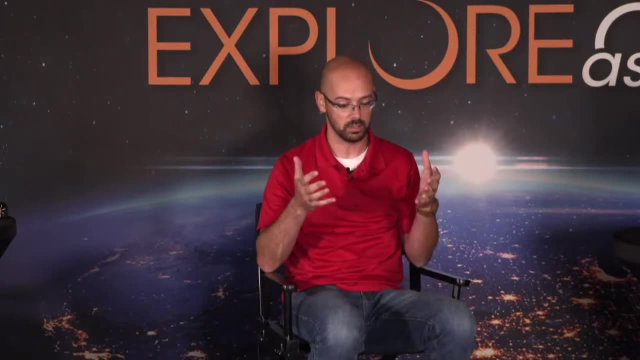 rover and sending it to Mars. Like you do kind of feel a little uneasy, but hearing all the safety precautions that you know INL and the Department of Energy have gone through to make this so safe, I feel safer. So thank you for talking to us about it. 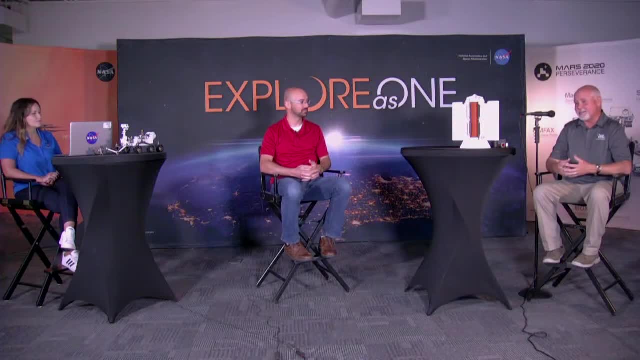 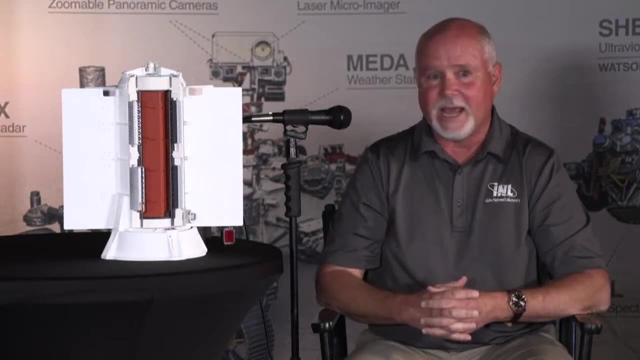 Absolutely So, And you know I can add too: I, you know I feel very safe around it. We work around this regularly at the Idaho National Lab. We've worked around it down here with NASA and JPL And in addition to the safety and the very rugged 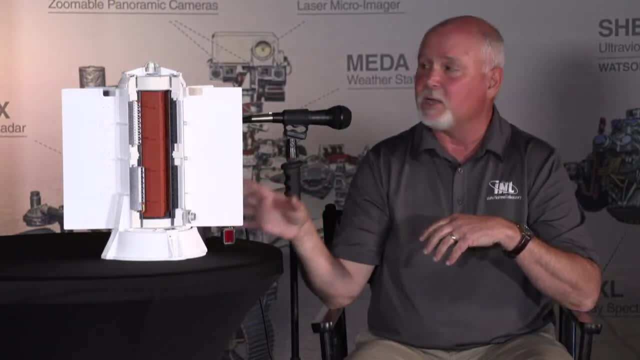 compact safety features and protective layers that the module provides, as well as the layers in the RTC. you know NASA has done a remarkable job of contingency planning And you'd have to talk to them, to NASA, to get more details on that. 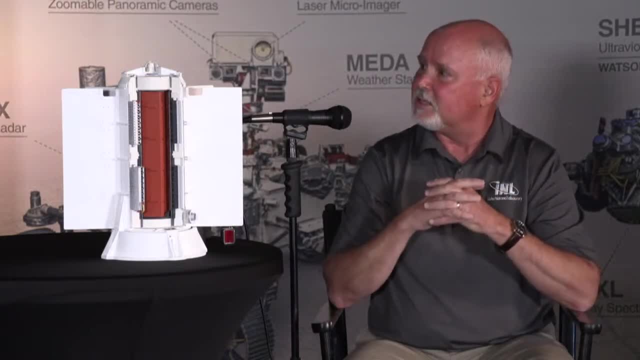 But that you know full on contingency plan in the event of an anomaly. Okay, Great. So, Allison, you said that was it for social questions. Yeah, that was all we have for social. Well then, I will ask my last question. 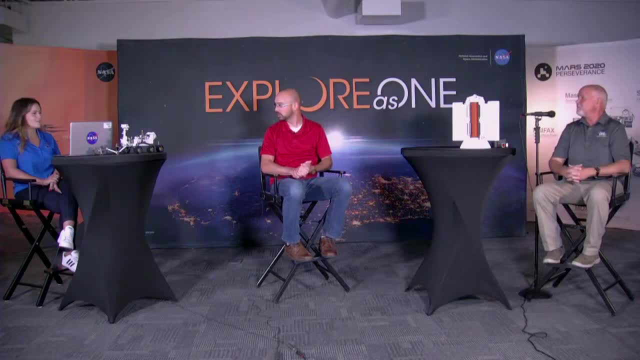 And that's Greg. where are you going to be for launch tomorrow? I will be in the Joint Information Center, which is part of the Radiological Control Center. So you know I'm going to be in the Joint Information Center. 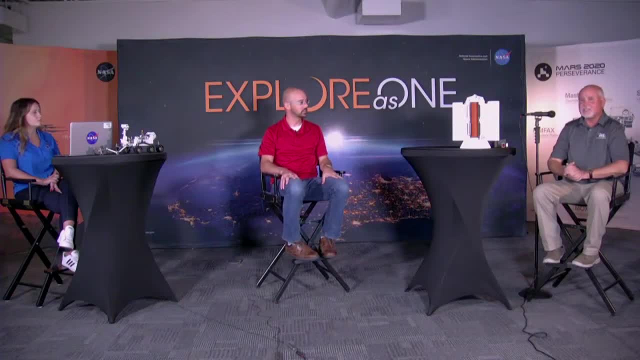 which is part of the Radiological Control Center. I'm going to be in the Joint Information Center, which is part of the Radiological Control Center. I'll be serving as the MMRTG point of contact during the launch. How exciting. I'm excited.